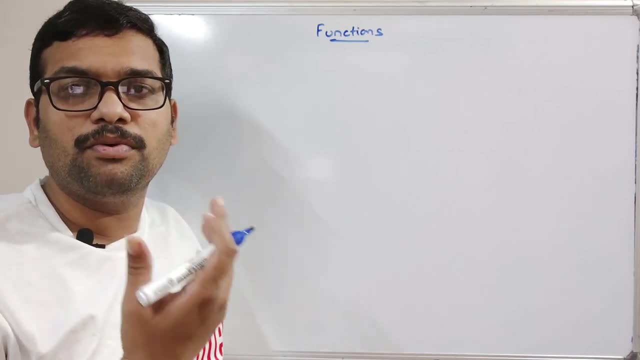 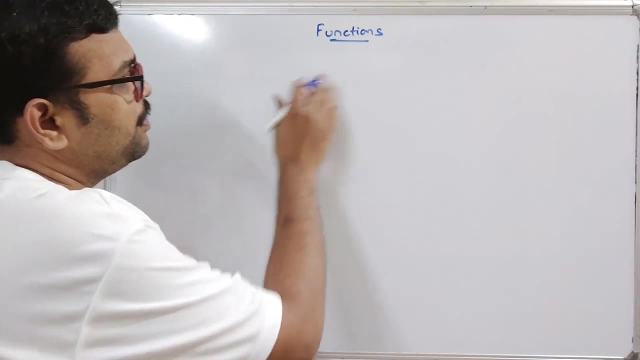 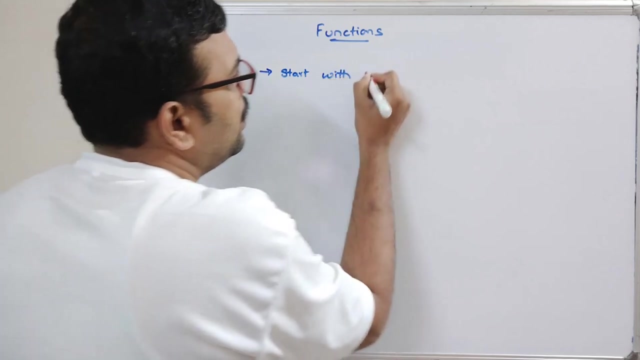 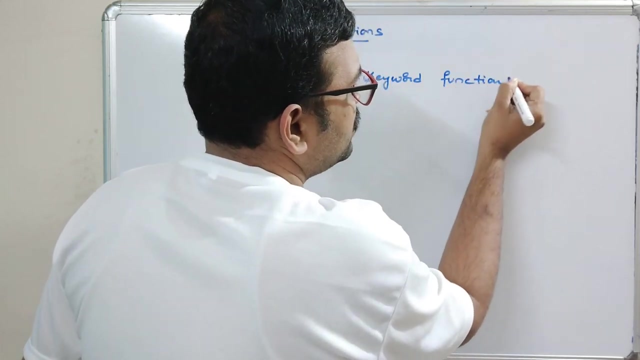 session we'll talk about the user defined functions, so how we have to write this user defined functions and how many ways we can execute this one right. so, first one, these user defined functions should start with a keyword called function, a keyword function. so all the user defined functions should be starting with a keyword function, right, and then 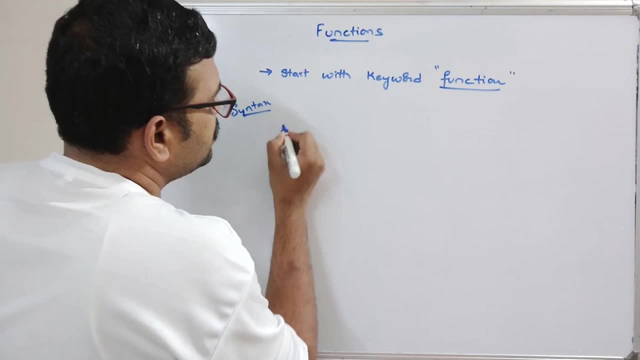 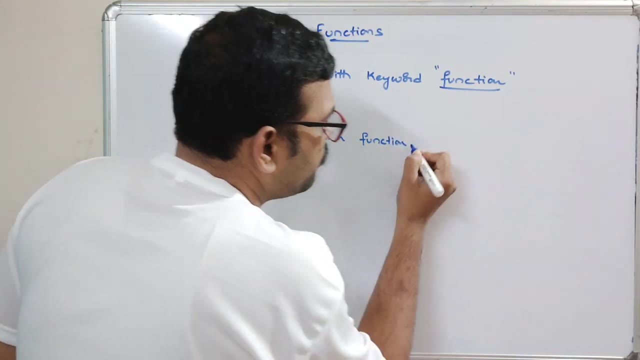 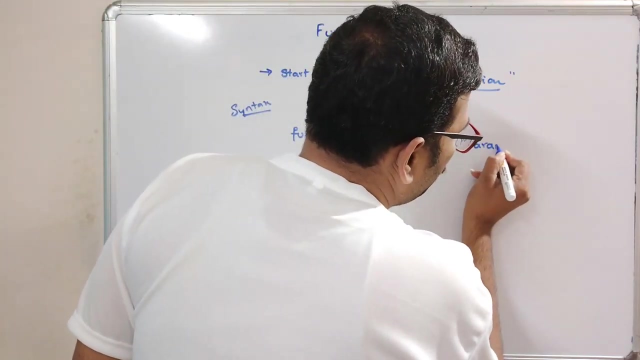 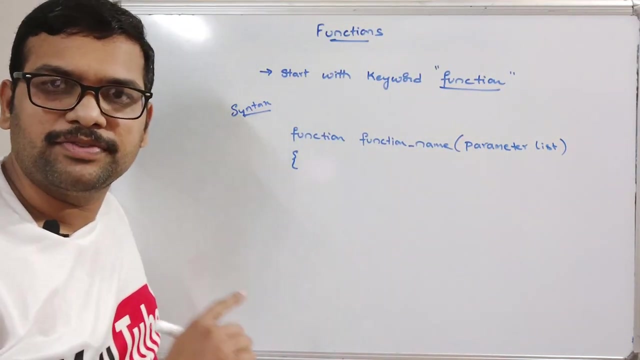 the syntax for implementing this function is function, so this is a keyword, followed by the function name. so for every function we have to give some a function name, followed by the parentheses followed by the parameter list. so here we have to pass the parameter list, so parameter list, and followed by the curly braces. it's a block of. 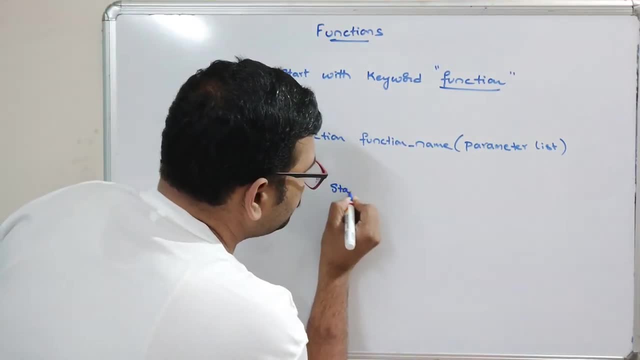 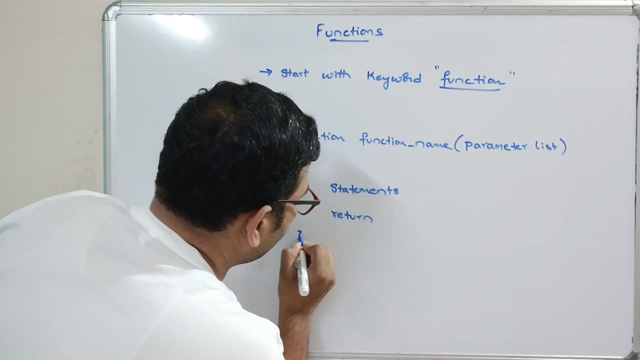 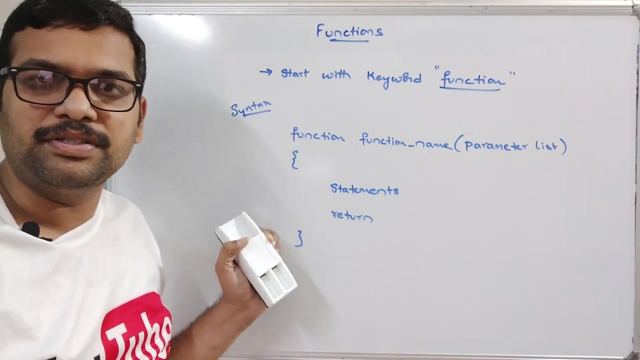 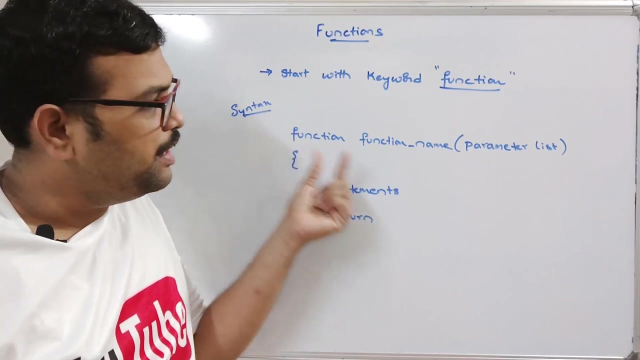 statements and here the statements, so, which we need to implement in this function. and then the return function, return type. okay, the return function, the return statement, and this is a prototype for implementing any function, so the function, followed by the function name. so this is a keyword. okay, this is a keyword and this is the identifier, so we have to follow the rules while 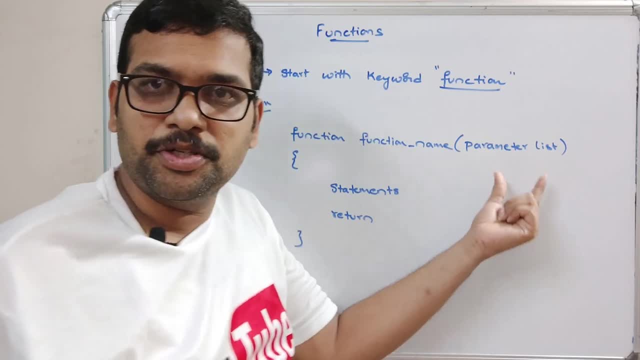 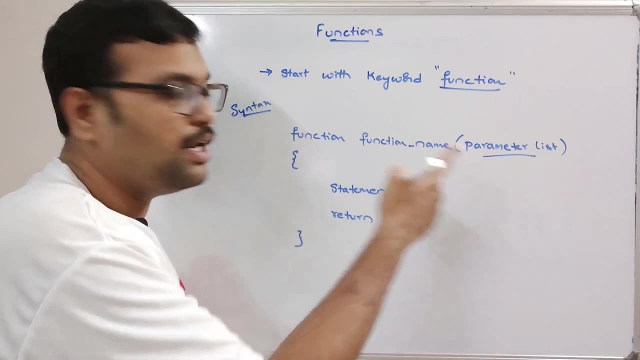 giving this name. okay, and coming to this parameter list, that is an optional, so we can give the input for this function in in terms of parameter list here, or we can also give the parameter list inside the function, right, and followed by the statements. that is a logic which we want to implement, and 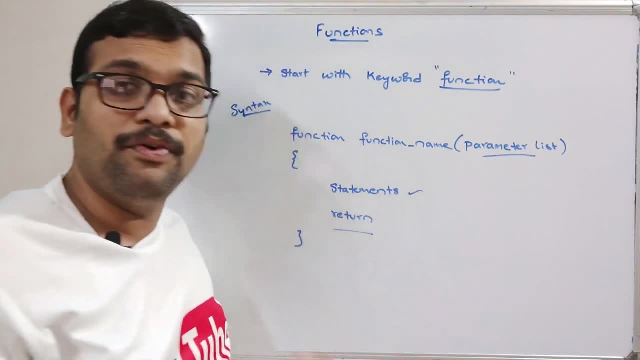 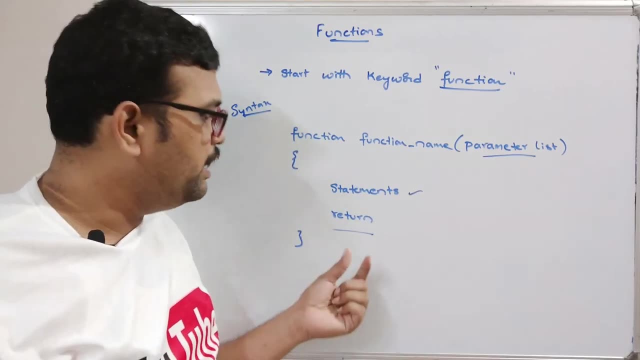 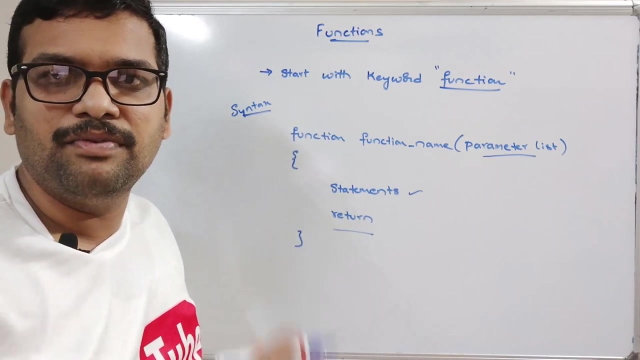 followed by the return. so this is also an optional. so if you want to return any value, then we have to go with this return statement. otherwise we can directly display the output here itself. okay, inside the function itself, now, when this function will be executed. when this function will be executed, so whenever there is a function call. 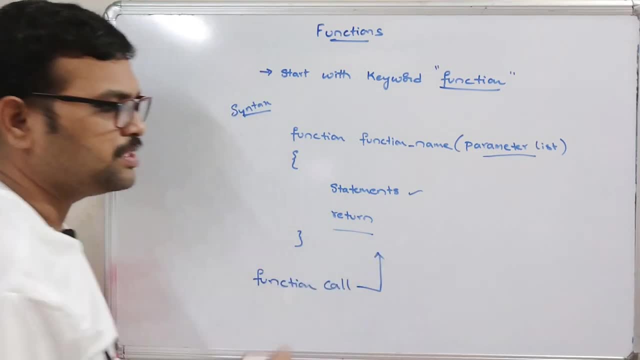 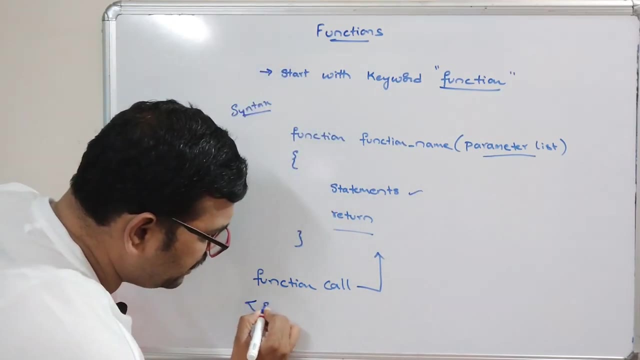 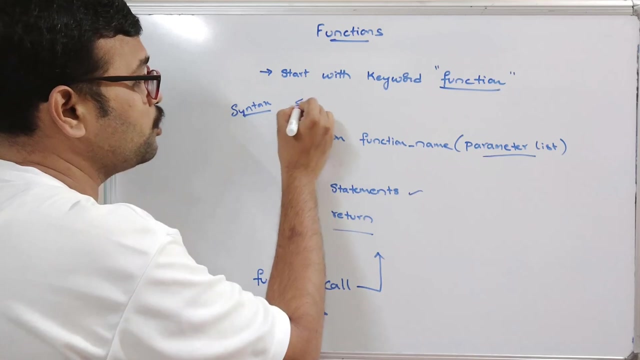 whenever there is a function call, immediately this function definition will be executed. and where we have to write this function call, and this function call should be written inside the script. okay, as well as this is once this is published. after these above must be each and whenever, in the description this: 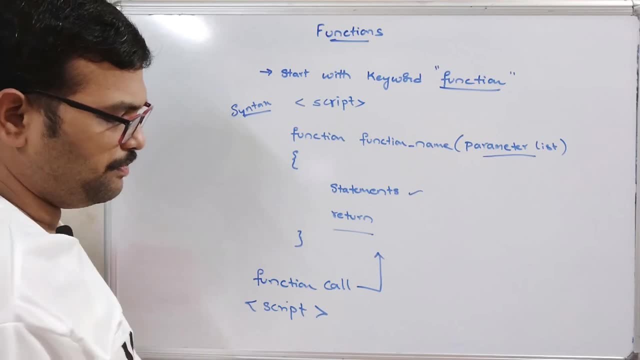 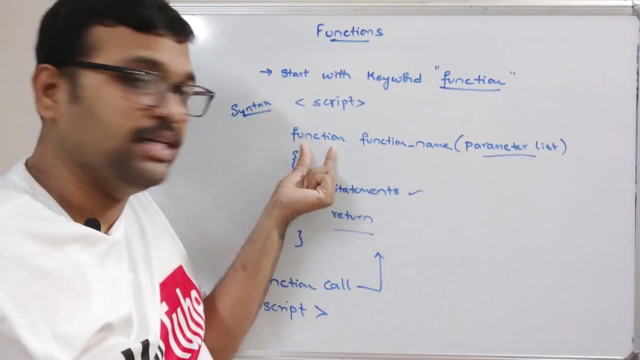 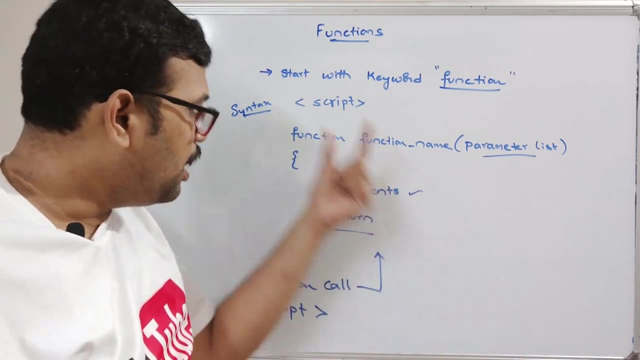 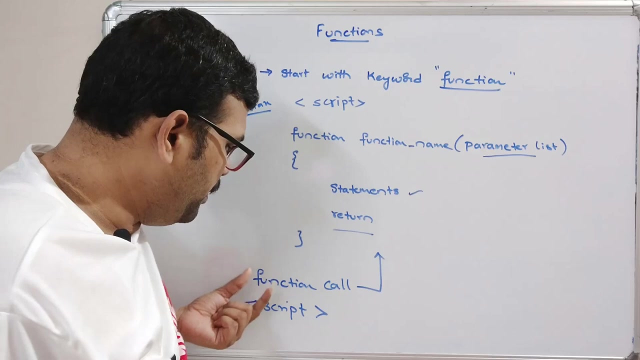 function definition should also be written in script tag itself. script tag itself, right. so whenever the control executes this one, whenever the control finds this function keyword, that implies this user defined function should be executed only after the function called. so automatically it will go for the next statement after compilation of this function definition. so 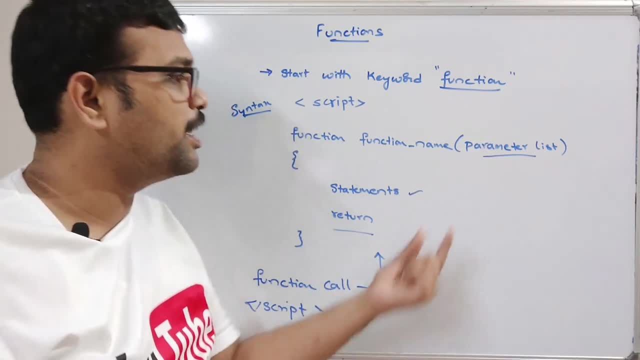 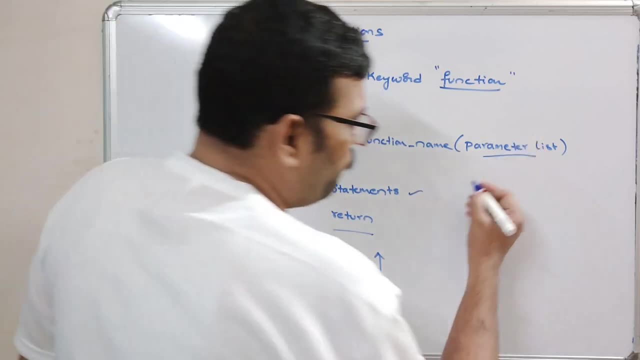 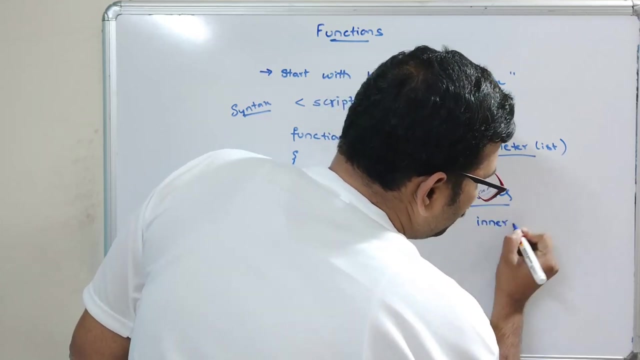 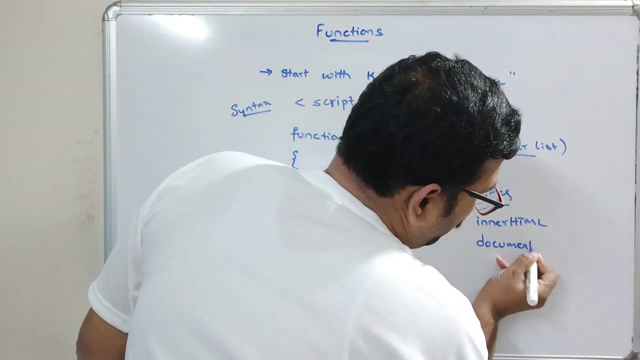 get the function call. whenever the control executes, this function call automatically finds for the function definition and this function definition will be executed and output can be written in a one among the three cases. so one is by using inner HTML. so we have seen this one right, inner HTML. and then document dot write. okay, document dot write as well as window dot. 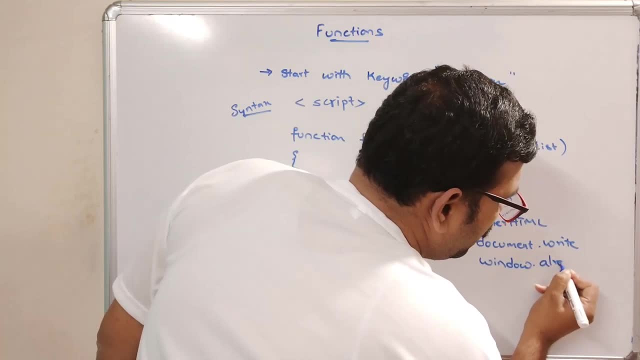 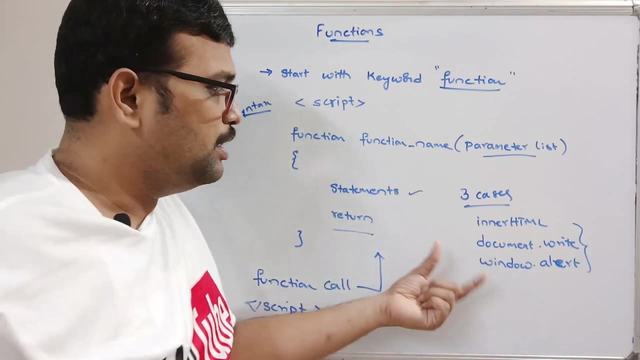 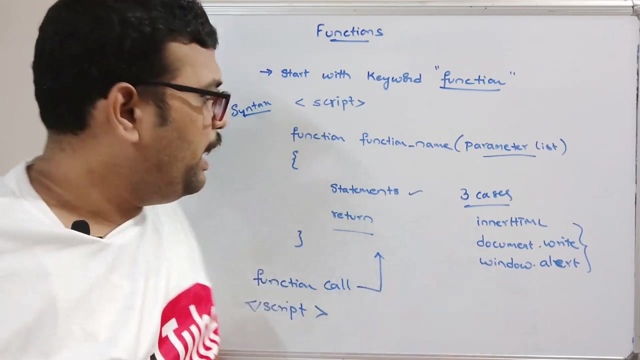 alert. so we also seen this one window dot alert. so we have to give the output. we have to display the output in one among these three categories. okay, we have to choose any one among these three in order to display the output and passing the parameter. that depends upon the logic, so we can. 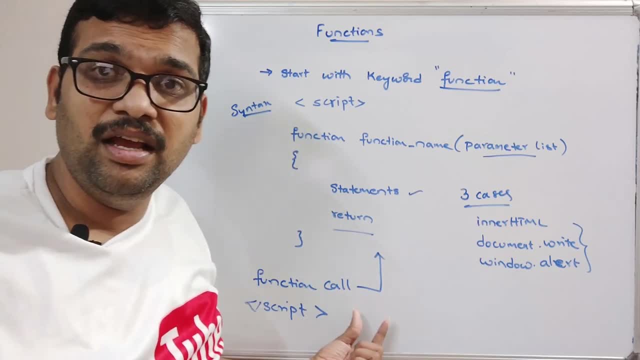 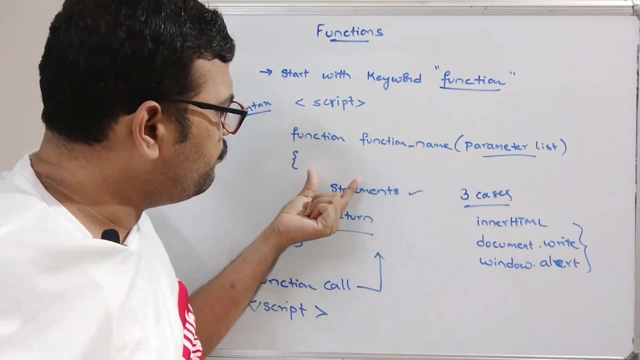 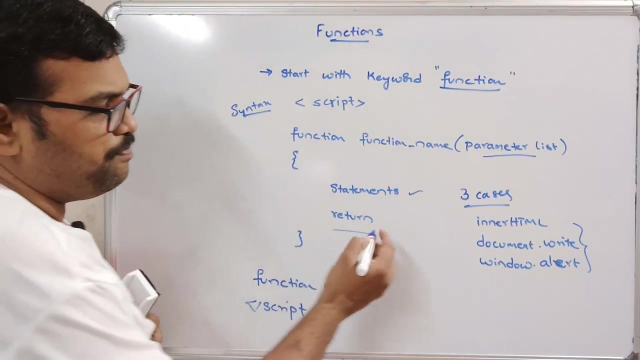 pass the parameter from the function call itself. so if you are giving any parameters or inputs in the function call, that should be reflected in this parameter list in the function definition. otherwise, simply, we can give the input inside the function call function definition also. and also if you want to print the result outside the function, you have to use this return statement. 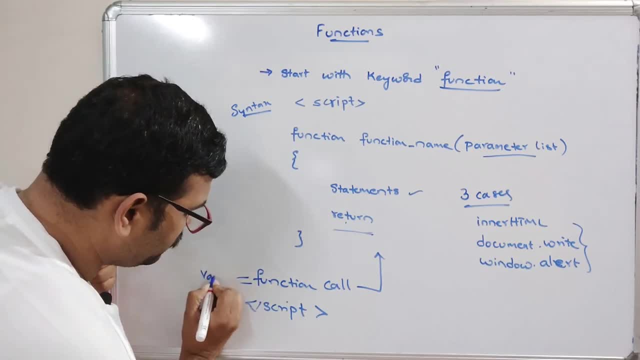 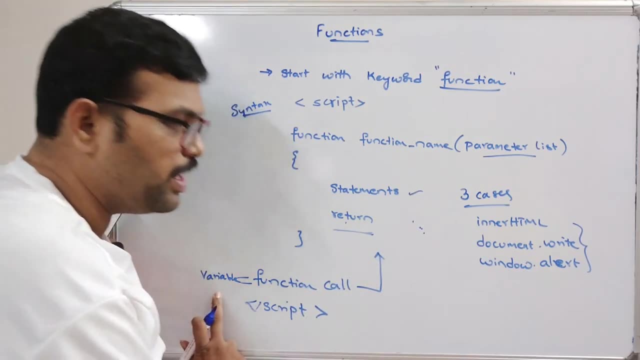 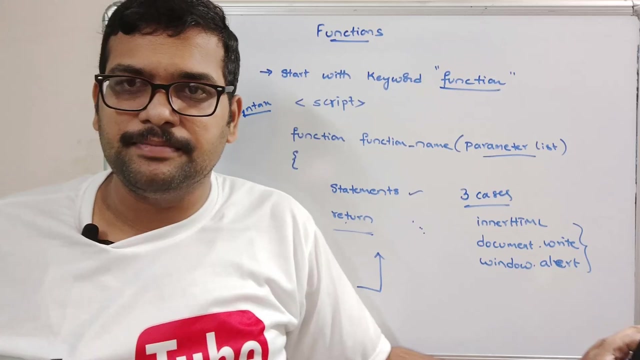 and that function call should be initialized to some variable and the result of this function definition will be stored in this variable, so that we have to display this variable by using one among these three things. these three functions: inner HTML or document dot write or window dot alert. right, so this is how we can implement the functions. okay, so one thing, we 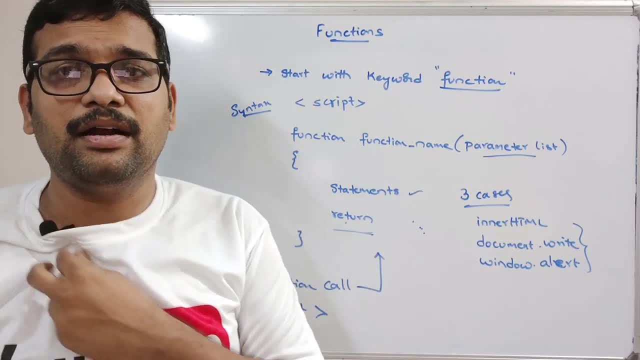 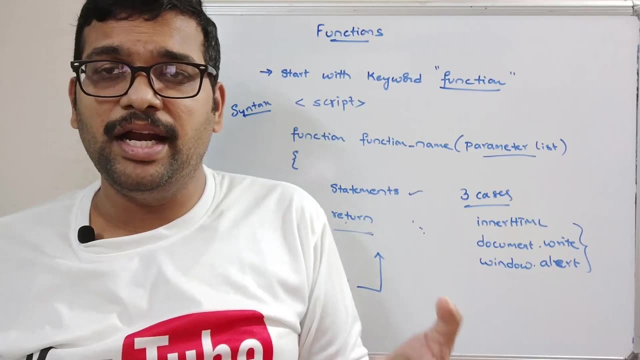 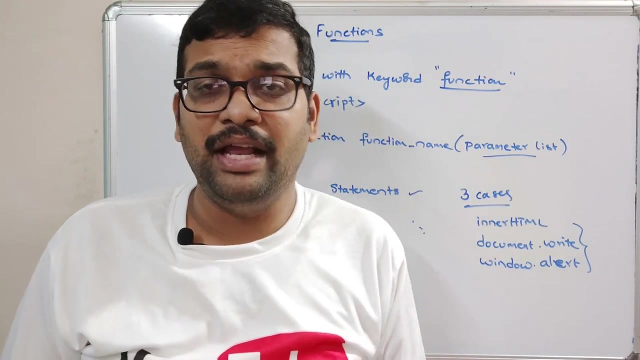 have to remember that is so. function can be written inside the script and we have already seen in the previous sessions that script tag can be included in inside the head tag or inside the body tag. so anywhere we can write the functions, anywhere we can write the script tag. 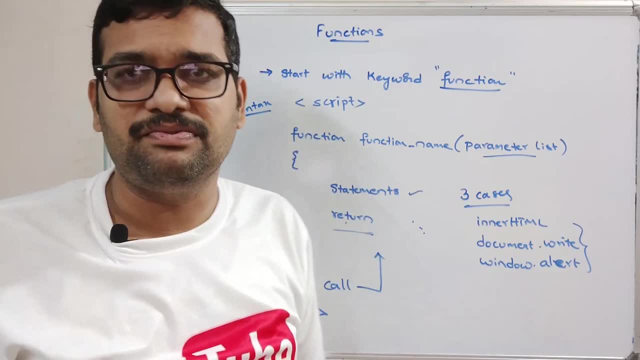 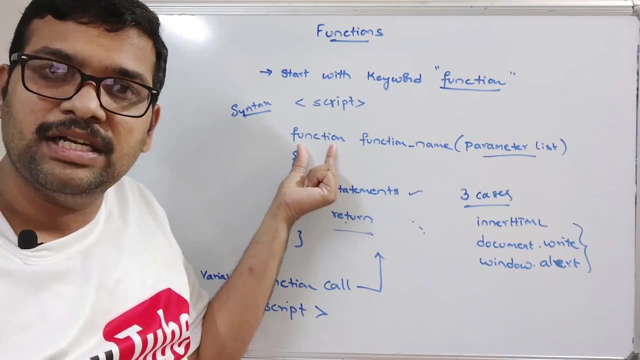 so inside the script tag, we have to write the functions and we have to implement the functions. these functions, right? So this is a prototype. once again, I am saying this function- user defined functions- should start with a function keyword, followed by the identifier name parameter list. 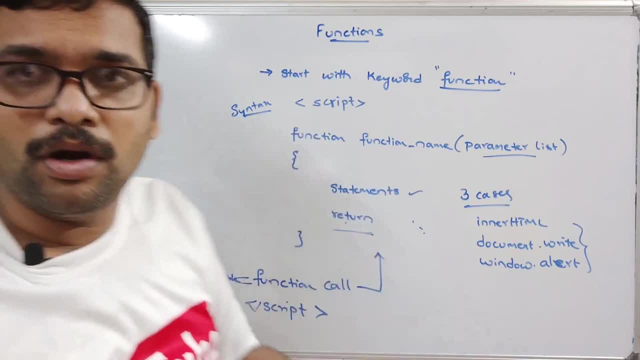 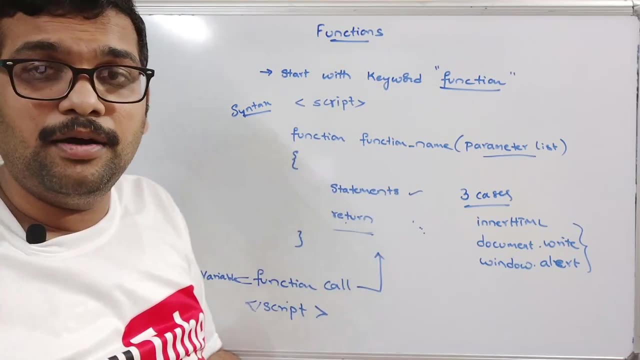 and the statements and the return right. So now we will move on to the computer. I will show you, I will demonstrate these function, how many ways we can implement this function and how can we display the output by using these three things. So all these things we will see by executing a. 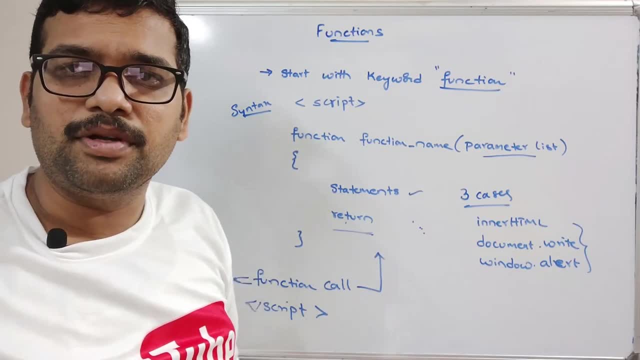 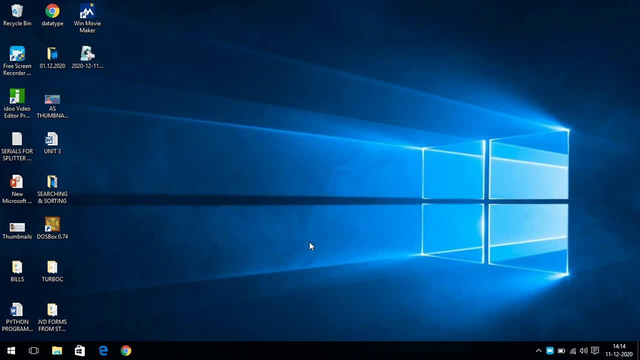 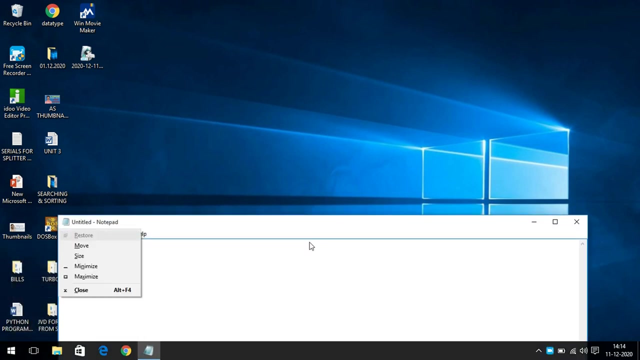 small HTML code, right, So let us move on to the computer. Hello friends, so just now we have seen the functions concept in JavaScript, So how to implement the function. So every function should start with the function keyword. So let's demonstrate that. the small HTML code. So. 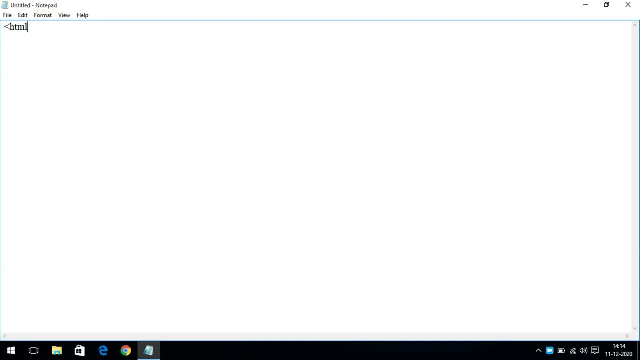 first we'll write the HTML tags. So inside the HTML I will write the complete function in this code. So inside the HTML I will write the complete function in this code. So inside the HTML I will write the complete function in this code. 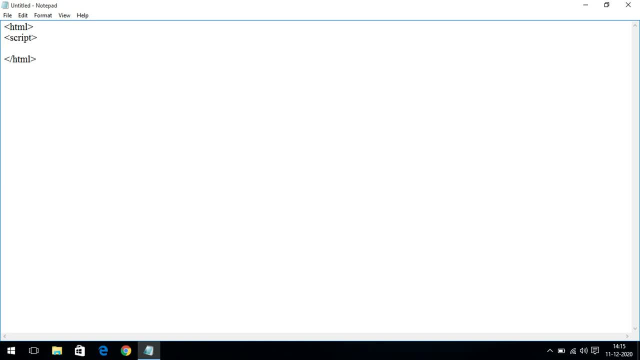 script itself. right, so we can write the javascript in either script tag or body tag. so i will write it in script tag. yeah, yeah, inside the script, first i will write the function. so every function should be starting with the keyword function function, followed by some add. okay, let us take some a. 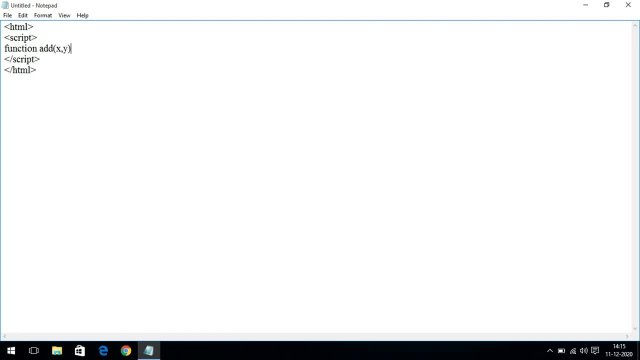 comma b or x comma y, x comma y and use the curly braces and here we can write the document. dot write x plus y, so x plus y. yes, so this we have written here and automatically, if this function is to be triggered we have to write some function call. so for that function call we can write here: 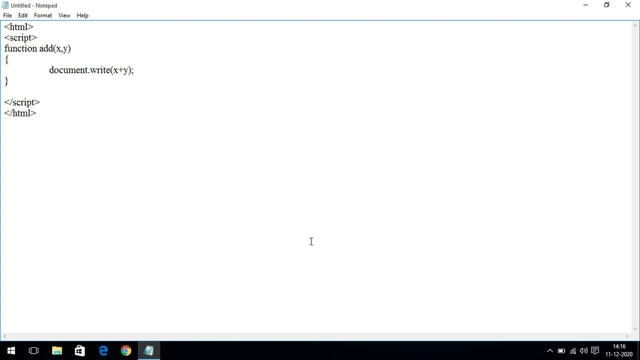 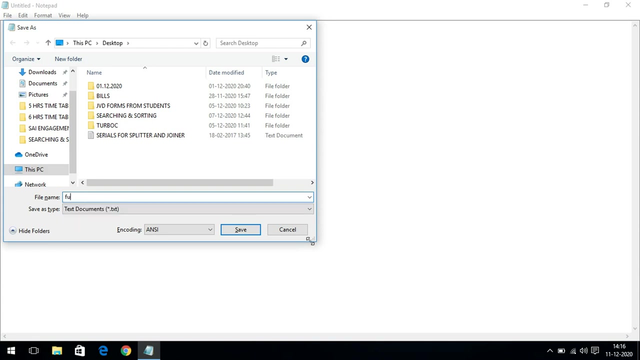 the function. we will take some variables where some a comma b and initialize some values- a is equal to 10 and the b is equal to 20- and write down the function. call right, add. add a comma b. right now, let us save this one with the help of one name: some. let us take some function. 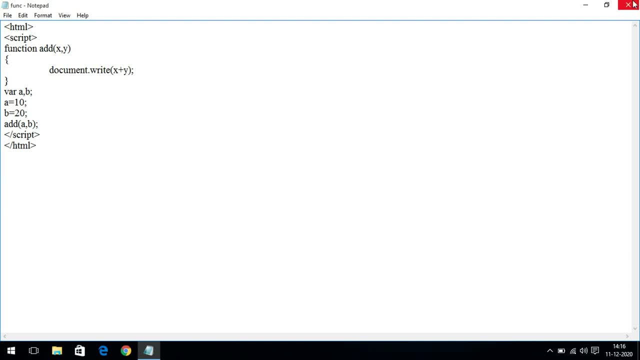 dot html. so i have saved this one in the desktop. so here you can see the file. so by double click on this one we'll get the result 30 right. so automatically, this function call will be so only whenever an event occurs. i mean whenever an event occurs or whenever the 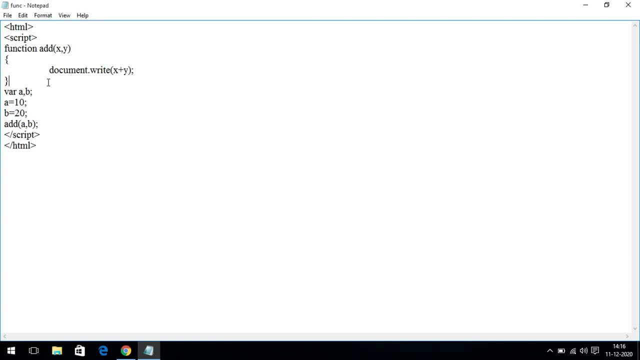 function call executes, then only this function definition will be executed, right? so this function keyword gives an idea to the javascript that this is a user defined function and that's a function definition and it should be executed only when the function call is executed. so here you can write. 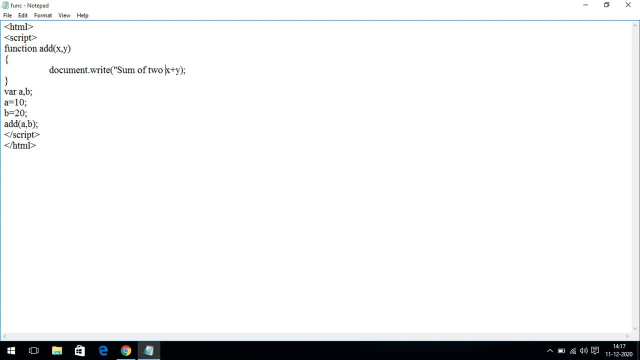 sum of two numbers is so that the complete content will be here. so you can also use the tags. here you can also use the tags. so with the help of tags you can write down here h1 and here you can close h1. see, this is how we can write. 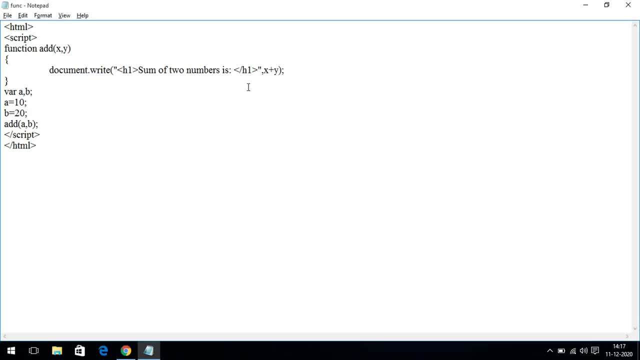 this one, and so this is the function definition with any return. so here we are not writing any return function, so directly we get displaying the output. but if you want to return some value, so here i will initialize the same thing to one variable right. so here i will give a, b comma sum. so sum is equal to a. add a comma b. 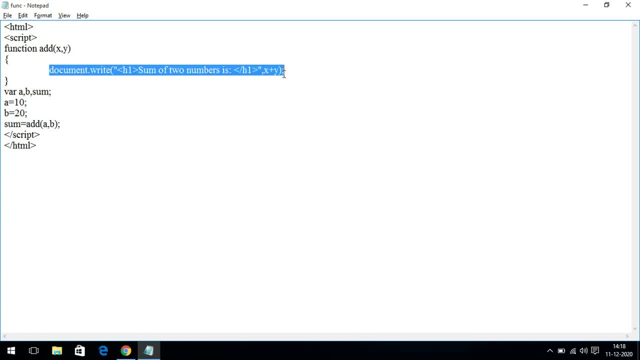 so that here we can't write this one so directly. we can write the return statement. so we will calculate the and we'll just return the addition here, x plus y. so automatically the result will be stored in sum, and after that we can write the result document dot. write, so not only by using the document dot. 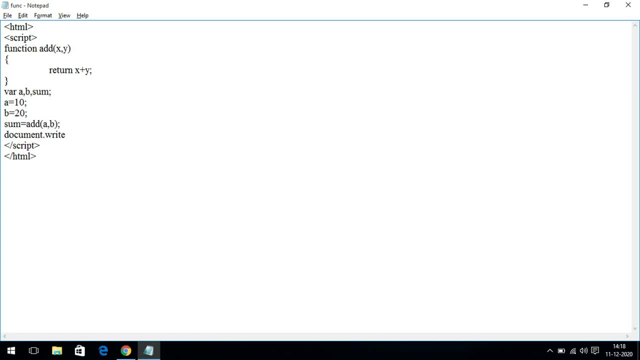 write. we can also use a window, dot lth or inner his table. so we have seen a different possibilities how we can display the output on the screen so we can use any one among those three functions, right, three categories. so by using document, dot write, or window, dot lth or inner his table. 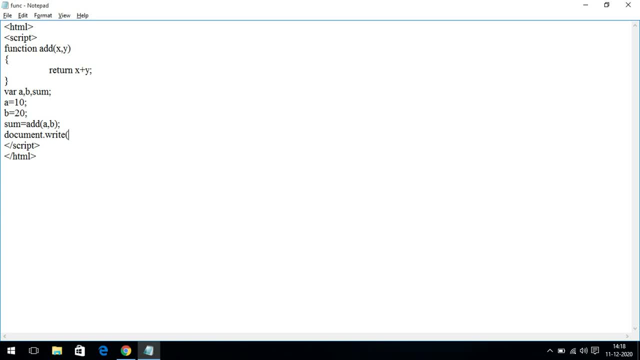 but here i'm using just document dot write. so document dot write, so you can write: sum of two numbers is and here we can give the sum, because so we are calling the function and the result will be stored in sum. so here we are returning the result, so automatically sum will be storing. 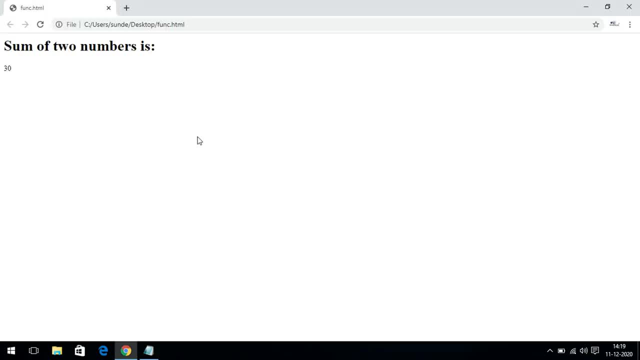 the result. so if you execute this one so automatically we'll get the same thing. see, sum of two numbers is 30. so here we are returning the result to one variable and that variable will be holding the result so that we can directly display that result here. 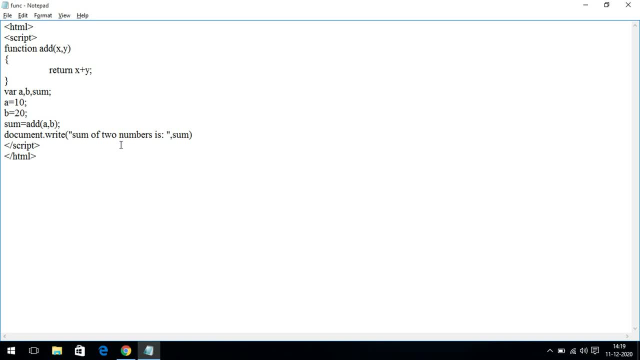 okay, this is one, this is another way. okay, so by using the return or directly, we can use that one and all these things. so instead of writing this one, we can also directly call here itself. so here, here itself, we can call the function add of a comma b. okay, so if you save this one and if you execute this one, so still, we'll get the. 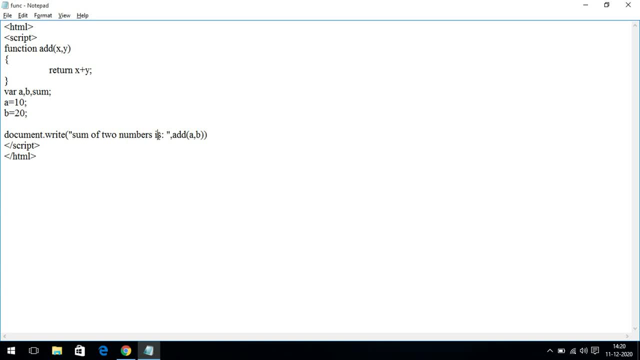 same result, right? so sum of two numbers is. so just will i will change the text. okay, so addition of two numbers is. now you can see the result: addition of two numbers. so we are not getting any error. so we can use the return and that return can be initialized to one variable and that variable will be holding the result and we can print. 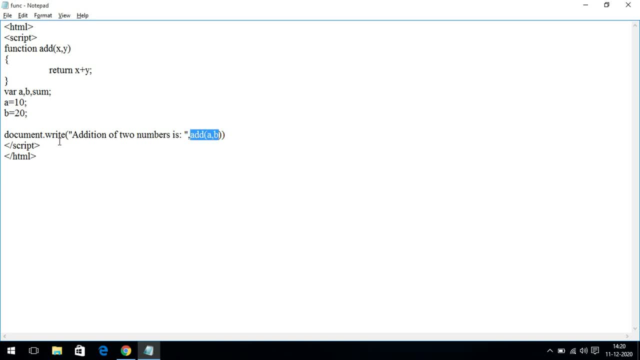 that variable or directly, we can use the function inside the output function, right, and this one. so with the help of this parentheses, the help of this parentheses, we can get the function definition. so another way, i will show you the another way. see, i'm not, uh, initializing here, just i'm going with. 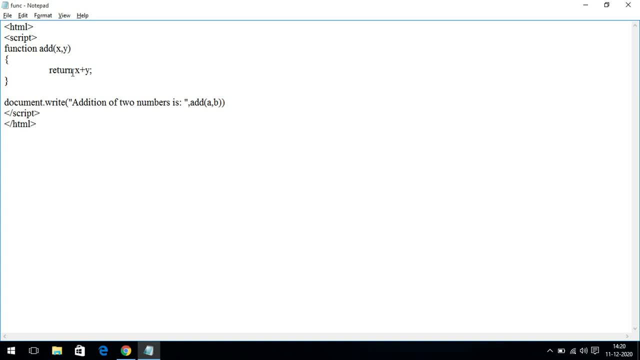 sum, or simply you can leave it, and here itself we can declare the variables a comma x, comma y, okay, and we can also initialize the values: x is equal to 10 and y is equal to 20, and see, here I will remove this one, also these parameters, and here also I will remove these parameters. 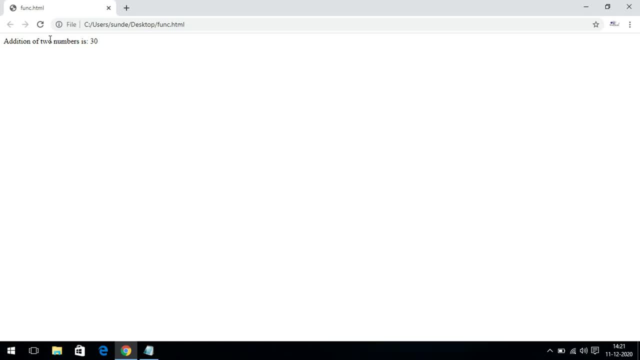 So if you execute this one still, we will get the same result. okay, still we are getting the same result because here, outside the function, we are not declaring any variables and we are not passing into the function call directly. we are declaring the variables inside the function. 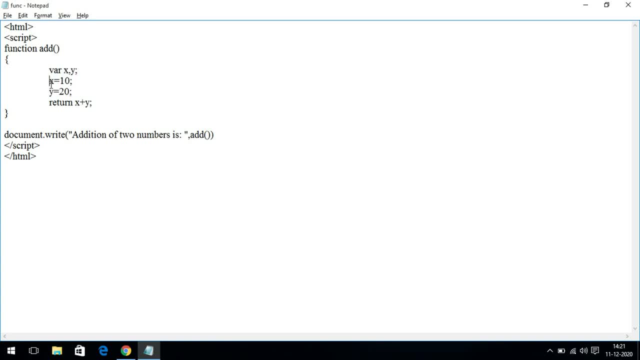 definition and also we are defining the values inside the function definition. So see, if you use these parentheses after this one, that gives the function definition, that gives the function result. if you are not giving these parentheses automatically, it will give the function object, see, So this is a function object. this is the function object we have written in the script. 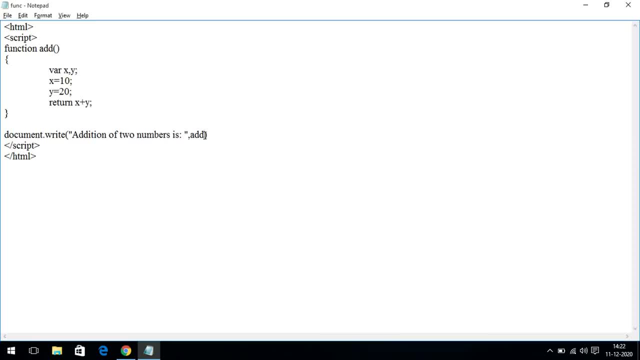 that will be returned if you are not using the parentheses. So this is a not using the parentheses for the function call. okay, So just I am using some add after that add. we are not using any parentheses, So that means it will return the function. object: the complete function. 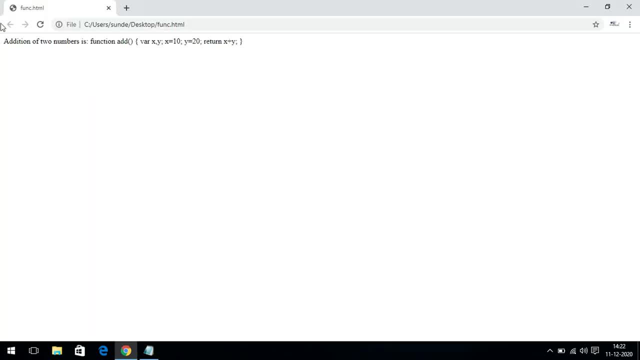 object and if you use the parentheses here, it will give the function Result. okay, see, you can observe the difference. addition of two numbers is 30, and, and the absence of this parentheses will get the complete function which we have written in the script tag. that is the one main thing. okay, that is the one main thing. and here, whenever we are, 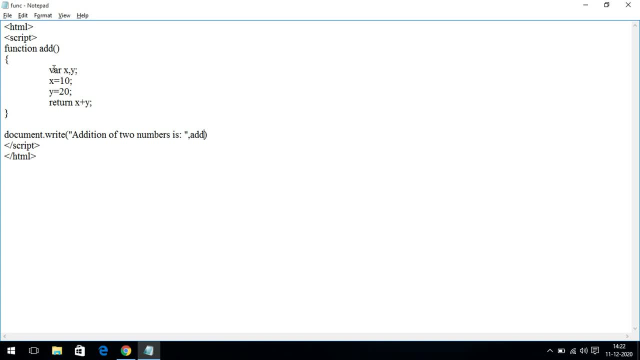 calling about this functions concept. So we have to know about the local variables and a global variables, and these variables, which are declared inside the function, will be treated as a local variables. this is how we can implement the functions in javascript. So hope you understood this functions concept. So if you are having any doubts regarding 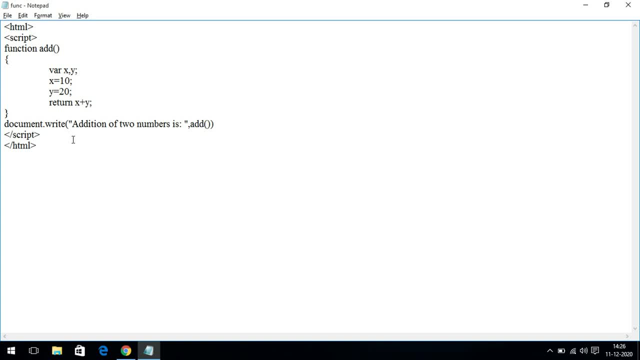 this function, implementing the function. So feel free to post your doubts in the comment section. So definitely, I will try to clarify all your doubts and also, if you really understood my session, like my session, share my session with your friends and do not forget to subscribe. to our channel. Thanks for watching. Thank you very much.